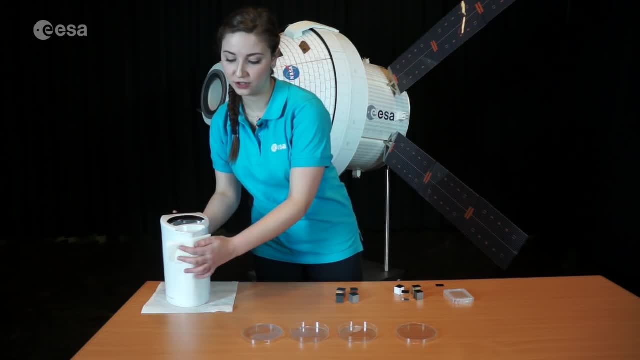 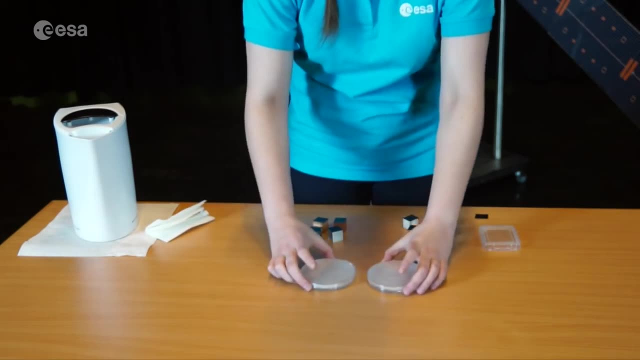 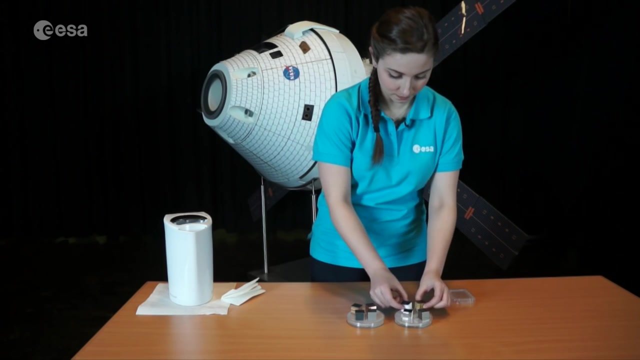 Next, very carefully, pour some hot water into each of the two petri dishes And cover both with the lids. Now take each of the cubes and place them on top of the petri dishes. You will notice the colour changes from black when the paper is cold. 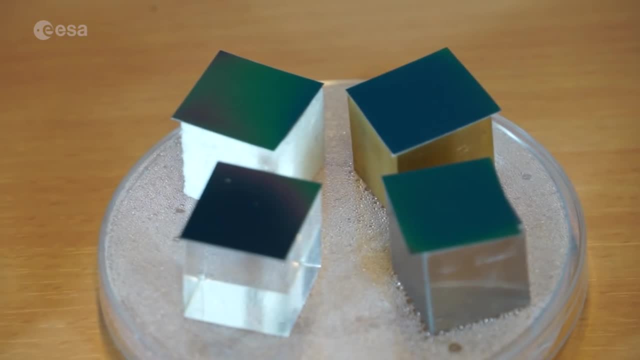 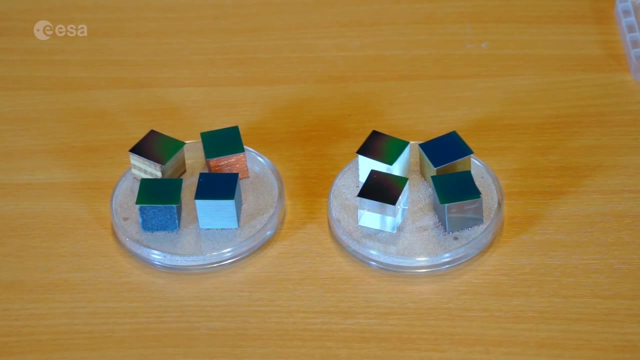 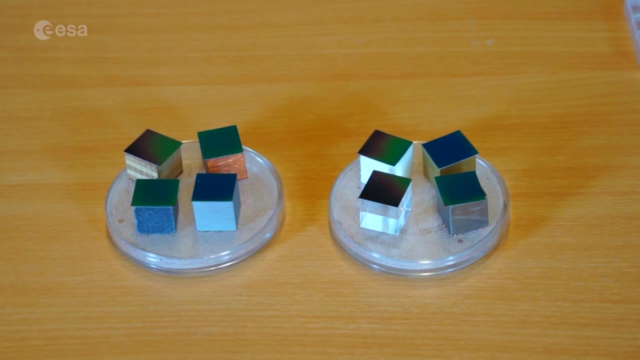 and as the cube begins to warm up, the paper changes colour to green. Pupils make note of which materials seem to conduct heat quickly By leaving the paper longer. they can also see which paper then begins to lose the heat, as it changes back to blue and finally to black. 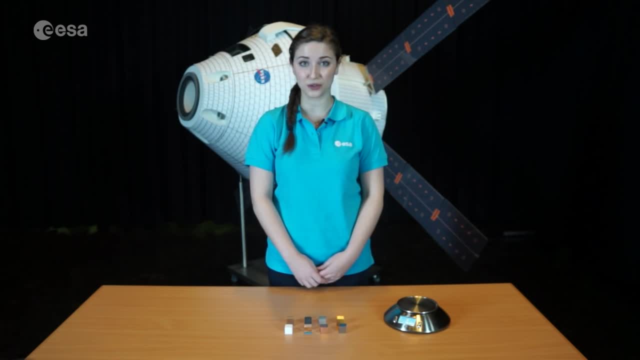 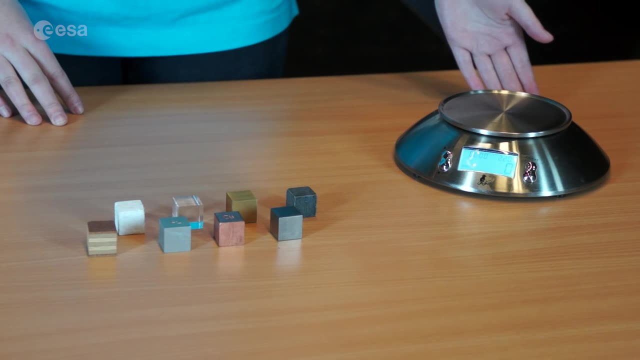 For this activity, we're going to be measuring the mass of each of the cubes. To begin, you're going to need the following materials: The eight test cubes and a digital scale. Pupils can begin by trying to estimate the mass to the nearest gram of each of the cubes. 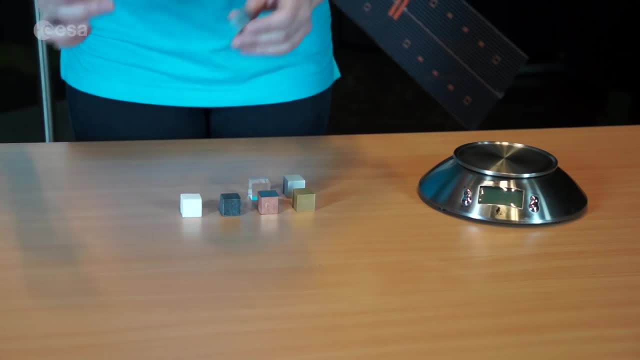 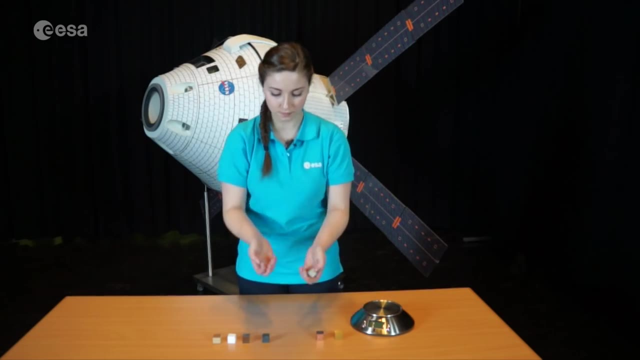 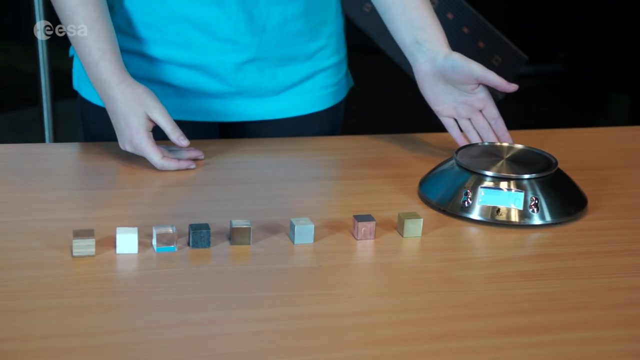 simply by feeling their weight in their hands. They can note down what they think is the heaviest and what they think is the lightest cube in their worksheet. Now that the pupils have noted down their estimates of each of the cubes, they can take an accurate measurement using the digital scale. 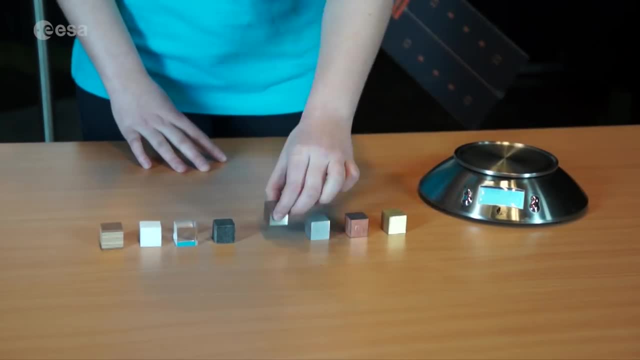 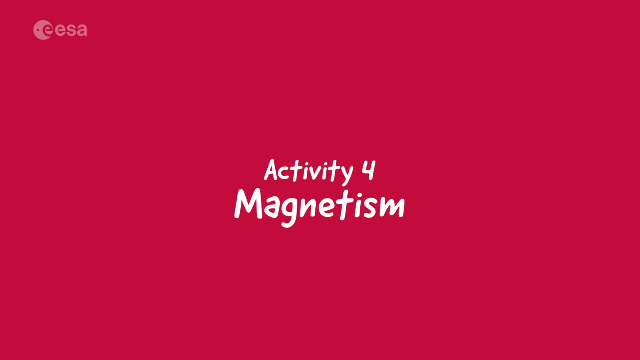 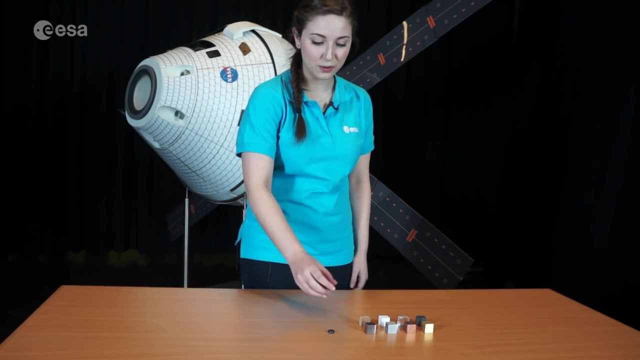 This measurement can be to the nearest decimal place. In this activity we're going to be testing which of the cubes are magnetic. You're going to need the eight test cubes and a magnet. Simply hold each of the cubes over the magnet to see if it's attracted. 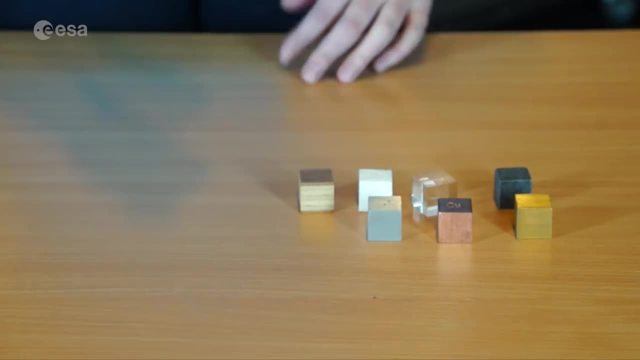 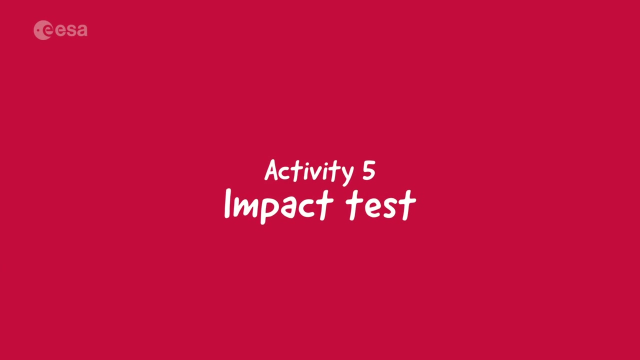 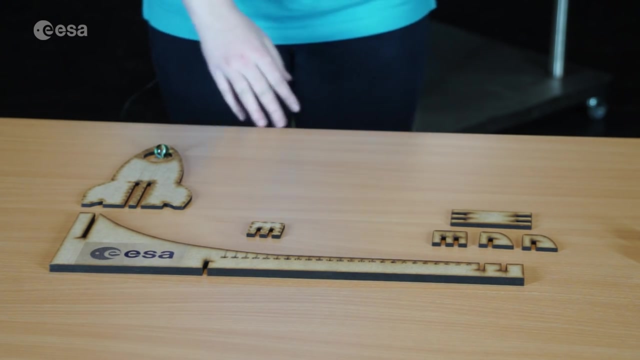 Pupils can write down if the test cube is magnetic or not. In this activity, we're going to be demonstrating the impact test. In order to do this activity, you'll need the following: The pieces for the ramp, the test cubes. 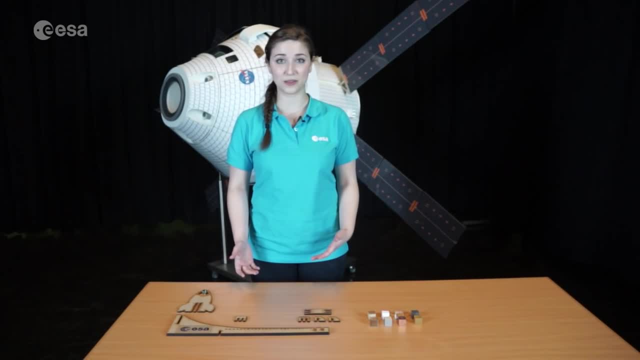 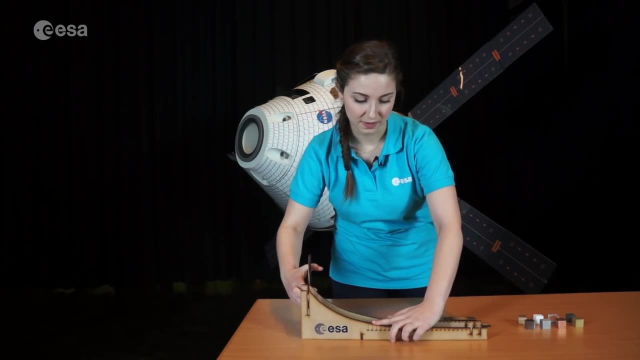 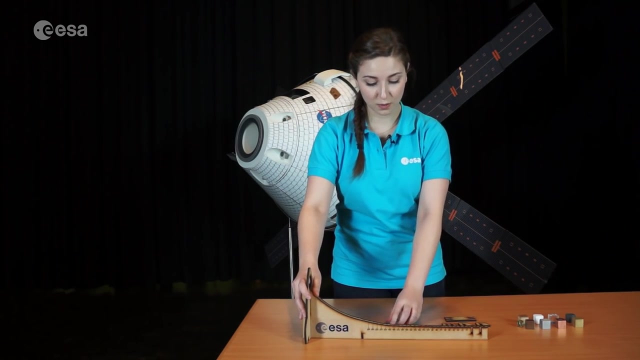 and a marble. First we need to start by assembling the ramp. Take the large rocket-shaped piece and slot it in to the top of the two ramp pieces. Next, take one of the E-shaped pieces and place that in the midpoint.